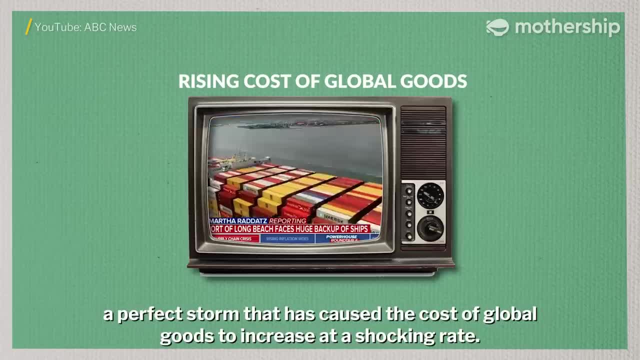 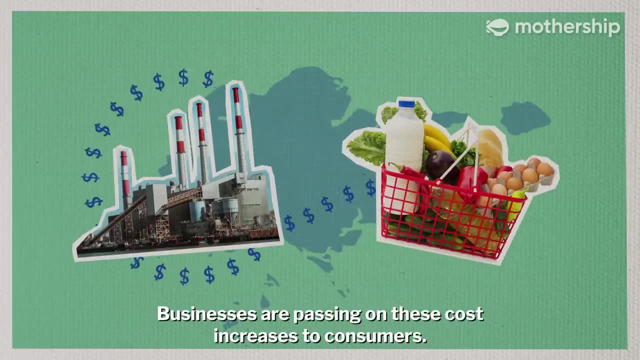 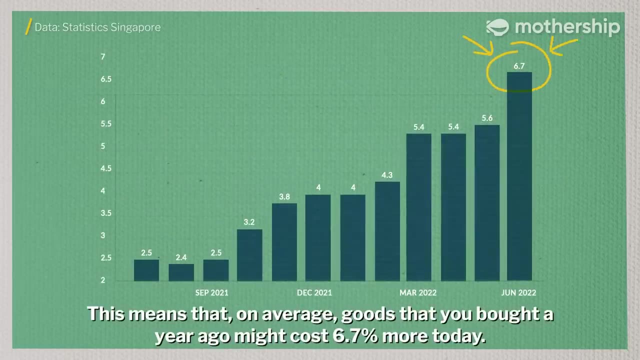 storm that has caused the cost of global goods to increase at a shocking rate. At the same time, the recovery in Singapore's labour market has resulted in higher wages. Businesses are passing on these cost increases to consumers. Just last month, overall inflation hit a 13-year high of 6.7%. This means that, on average, 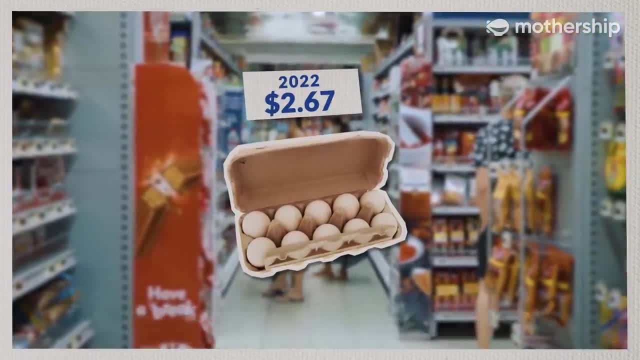 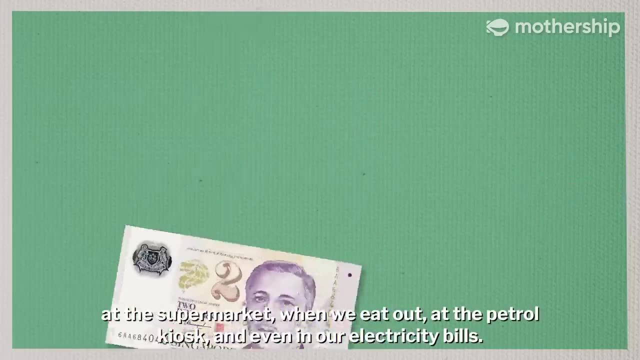 goods that you bought a year ago might cost 6.7% more today. We see signs of higher inflation nearly everywhere: At the supermarket, when we eat out at the petrol kiosk and even in our electricity bills. But a stronger currency means that Singaporeans have been protected from the worst of the global price increases. Suppose we want to buy an apple, The apple probably is imported from, say, New Zealand. So that means that Singapore is going to be a global currency. So that means that it has to be paid in New Zealand dollar If Singapore dollar gets stronger against the. 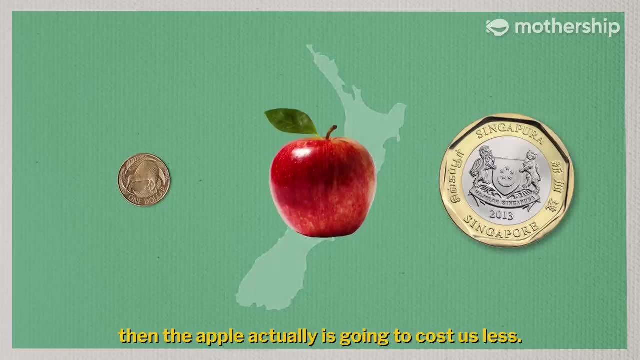 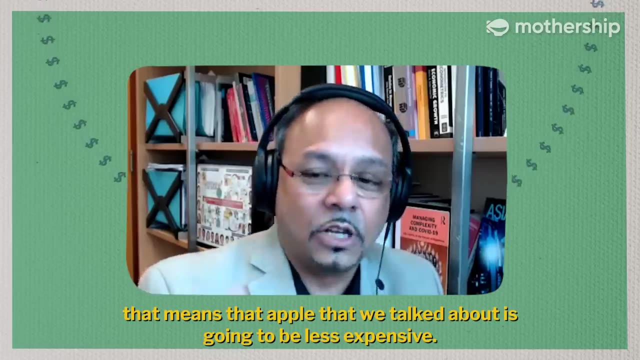 New Zealand dollar, then the apple actually is going to cost us less. If MS tightens the monetary policy, the exchange rate can be made steeper. That means that apple that we talked about is going to be less expensive. It cannot solve the problem completely, but it actually. helps somewhat. Over the past year global food prices have risen by about 23%, But in Singapore they have risen by 5.4%. But there are also costs involved with having a stronger currency. At some point. MAS can't keep pushing the Singapore dollar higher without growth slowing. 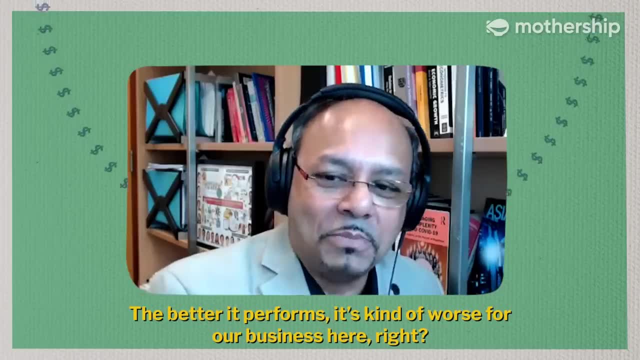 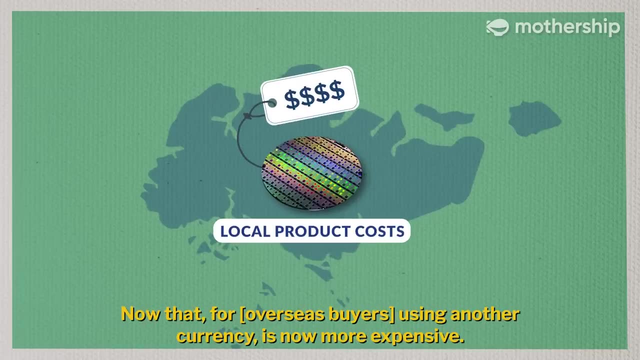 The better it performs. it's kind of worse for our business here, right? Suppose we are producing something like the silicon wafer for computer chips Now that for the other currency is now more expensive. The second thing: that Singapore wants to become a hub for financial technology. 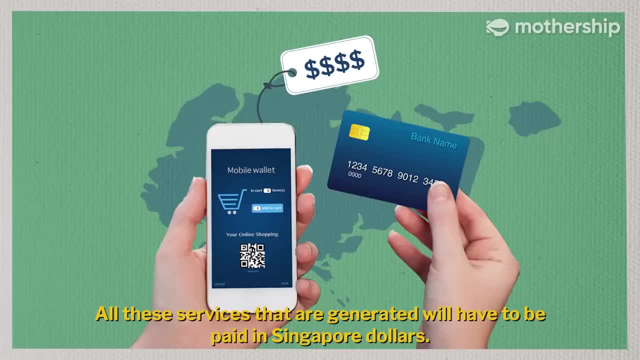 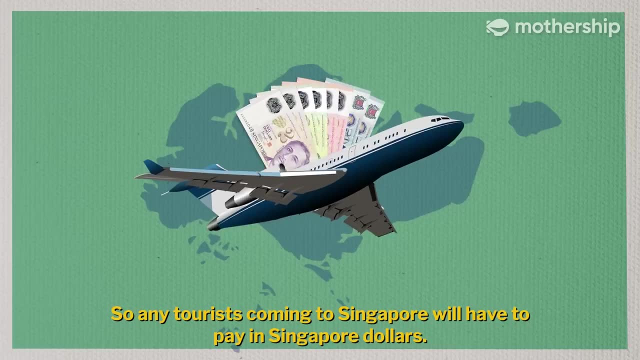 as well. All these services that are generated will have to be paid in Singapore dollar. So the service sector cost will also go up. I mean, last but not the least, tourism. So any business coming to Singapore will have to pay in Singapore dollar, If Singapore dollar appreciates. 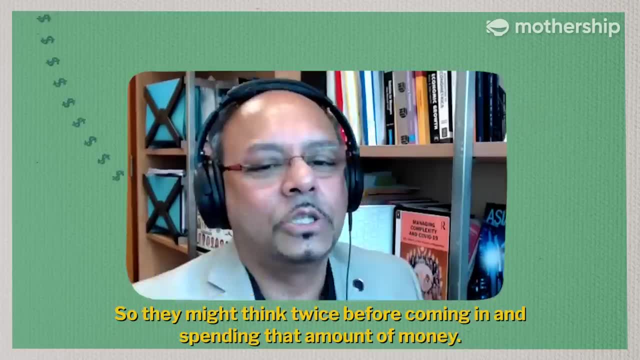 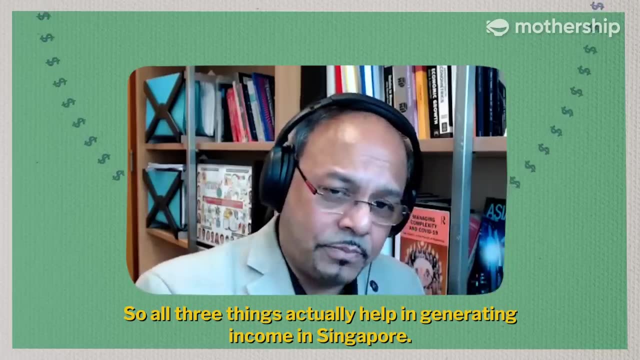 it is going to be a much more expensive vacation So they might think twice before coming in and spending that amount of money. So all three things actually helps in generating income in Singapore. There is kind of a fine balancing act, Even though the stronger Singapore dollar has. 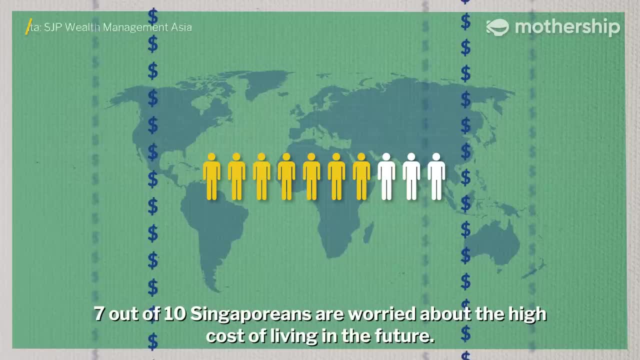 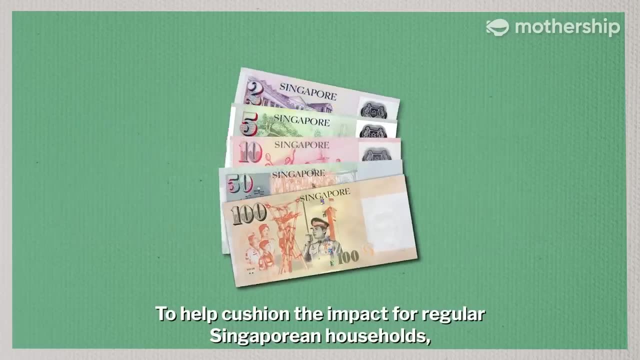 cushioned some of the impact of higher global prices. 7 out of 10 Singaporeans are worried about the high cost of living in the future. However, there are government support schemes available to help you. To help cushion the impact for regular Singaporean households, there are short term subsidies such as $100 CDC vouchers.